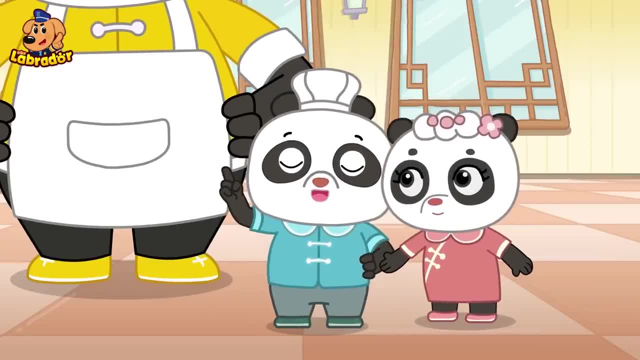 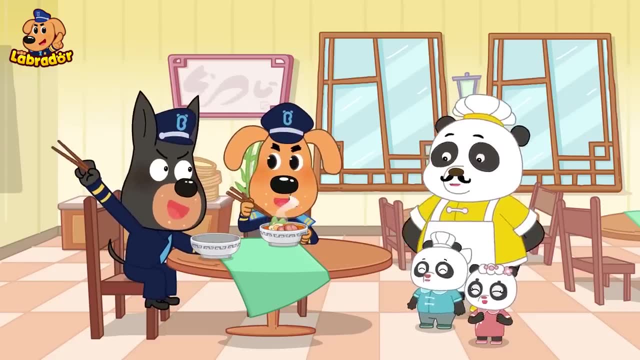 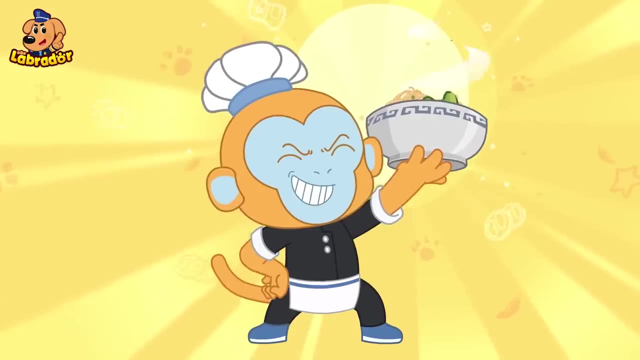 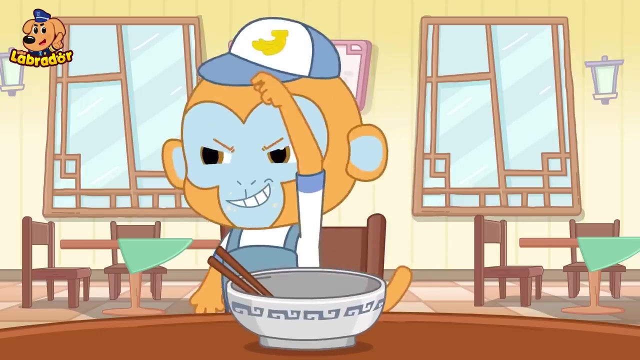 Secret spice mix. Yeah, the recipe's from our daddy's, daddy's daddy. That's right. Another bowl, please. If I had the secret spice mix, I'd be able to make yummy noodles too. Amazing, Amazing, Amazing. 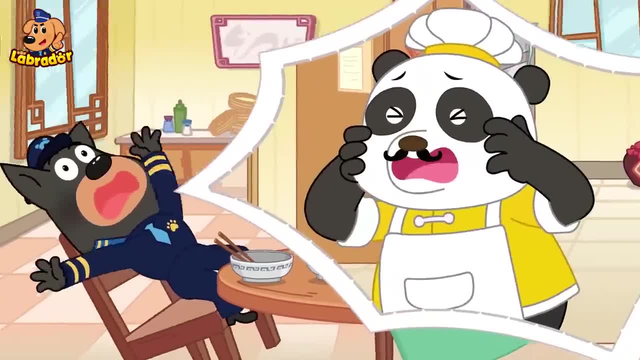 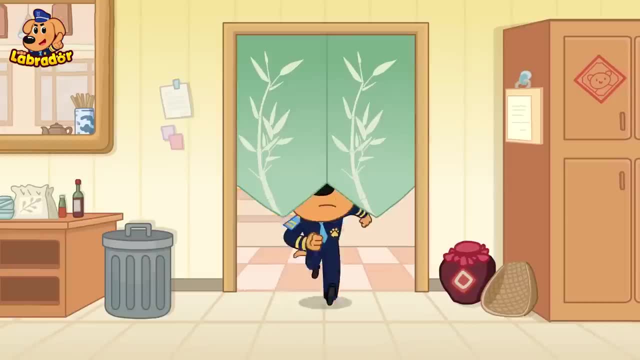 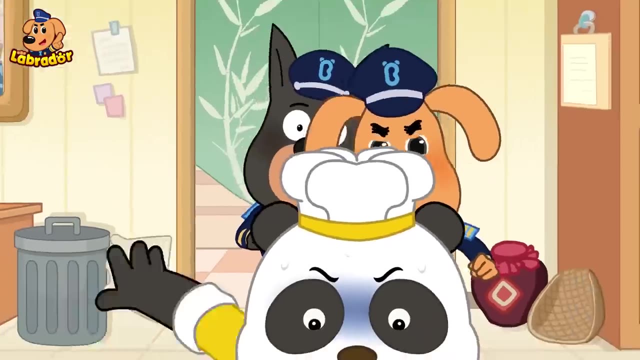 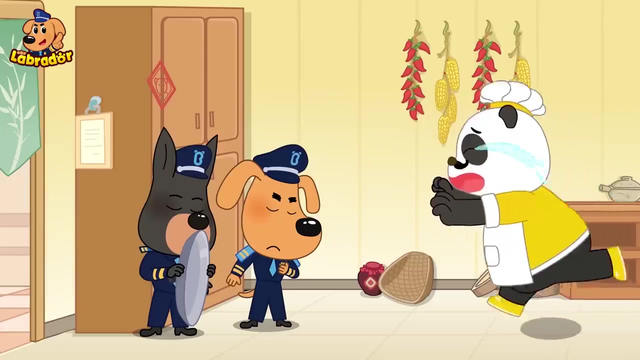 Another bowl please, Mr Panda, My spice mix. What happened? Let's go and have a look, Mr Panda. what's wrong? Sheriff Labrador, my secret spice mix is gone. What, What? It's handed down to me by my family and now it's gone. 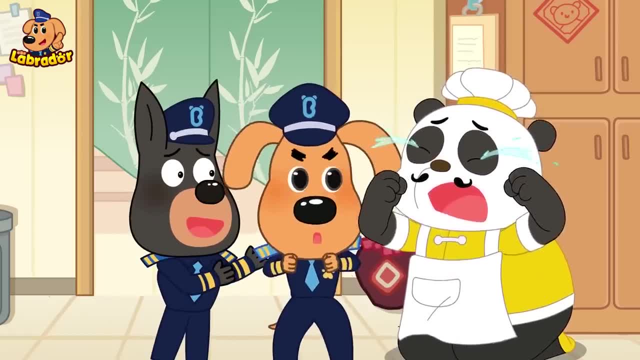 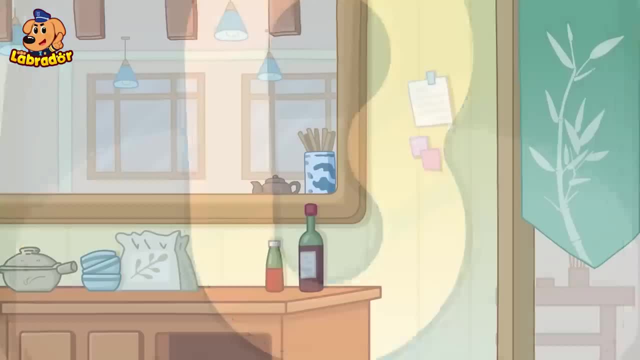 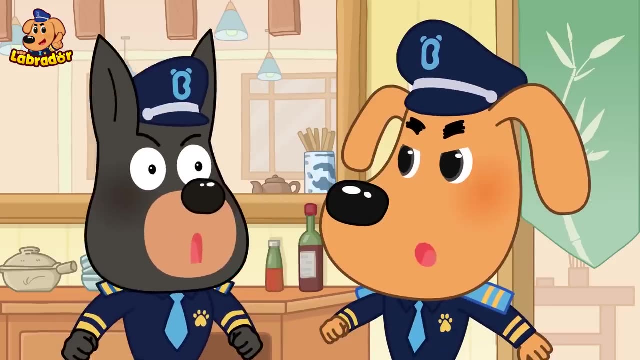 Please help me find it. Don't worry, There's no case that I can't solve. If it was stolen, there must be clues left around here. Dobby, let's split up and look around. Hmm, Hmm, Hmm, Hmm. 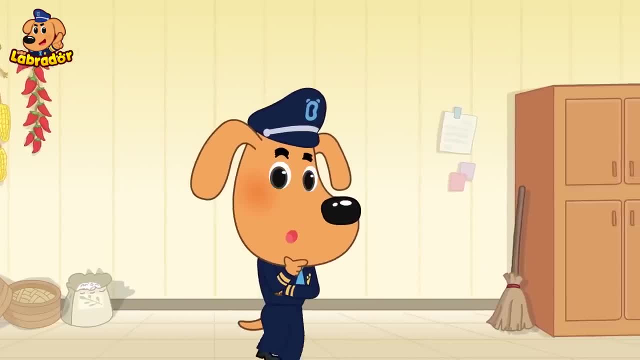 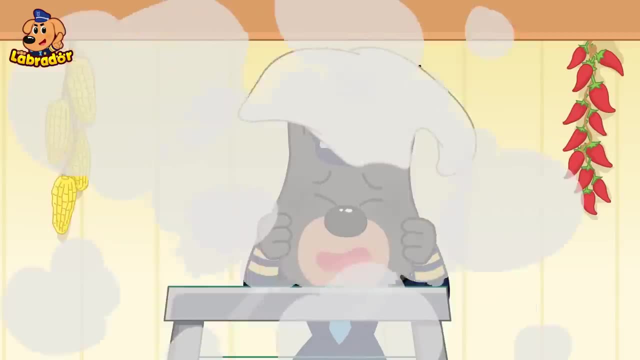 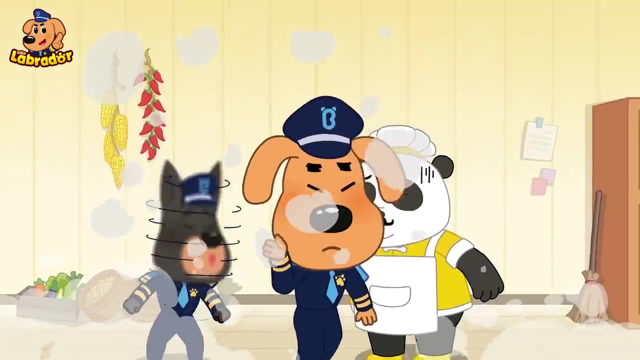 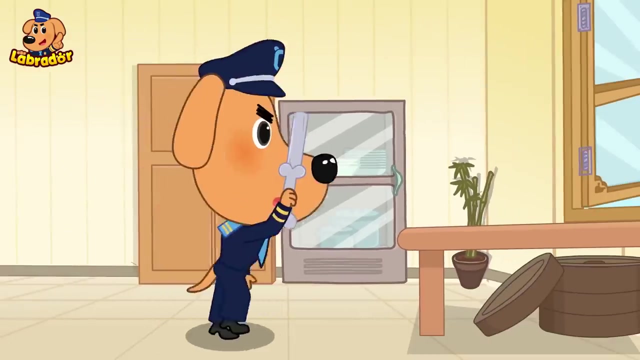 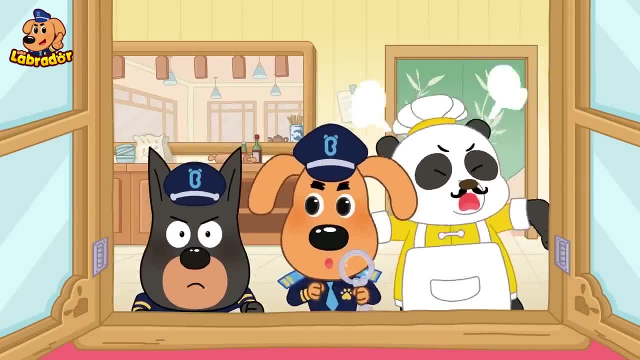 Huh, Unbelievable. I'm gonna catch the thief. The thief might still be here. What Look? there are no footprints leading out of here, So the thief must still be here. You can't run away. I got you. 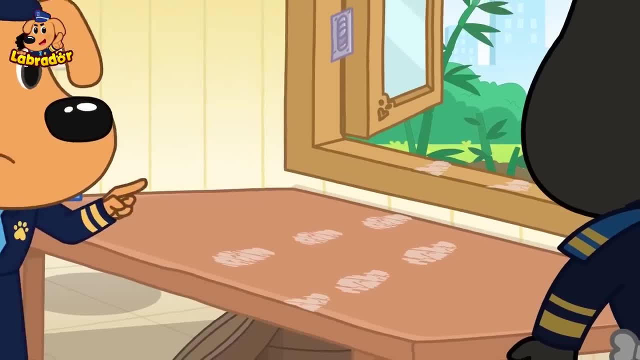 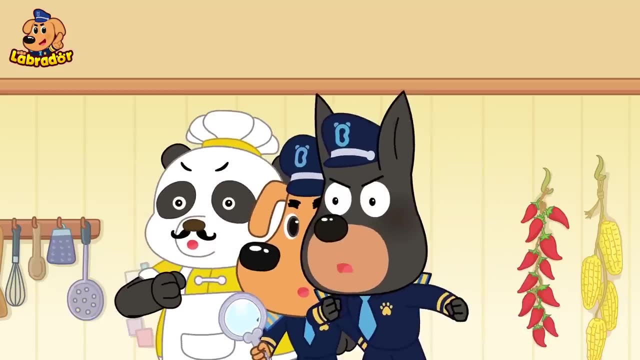 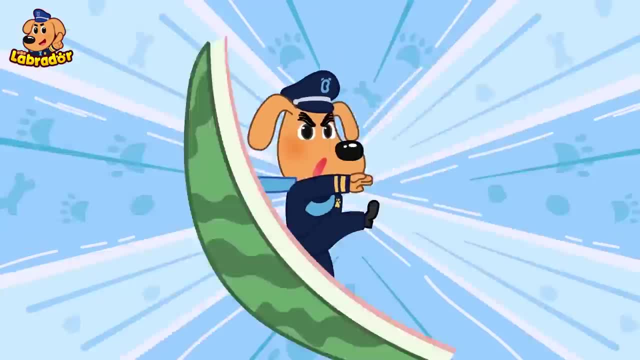 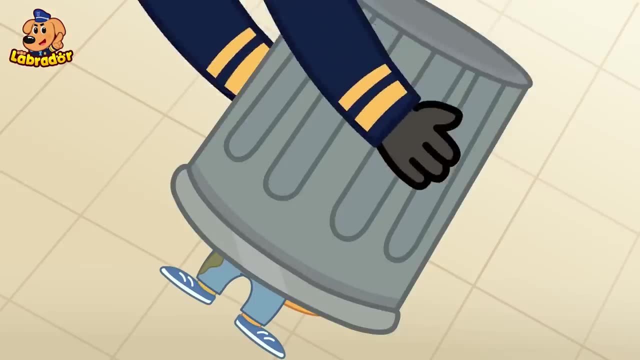 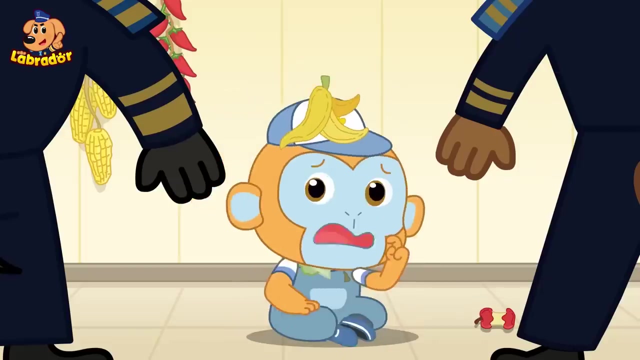 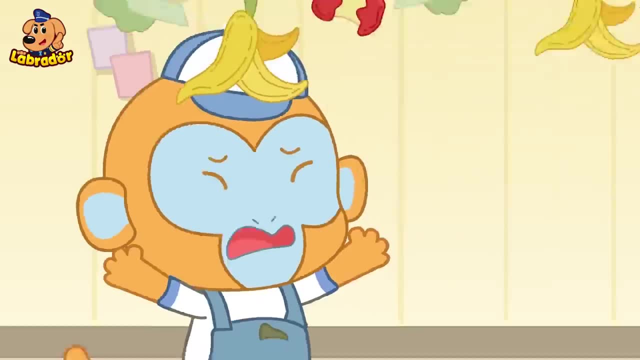 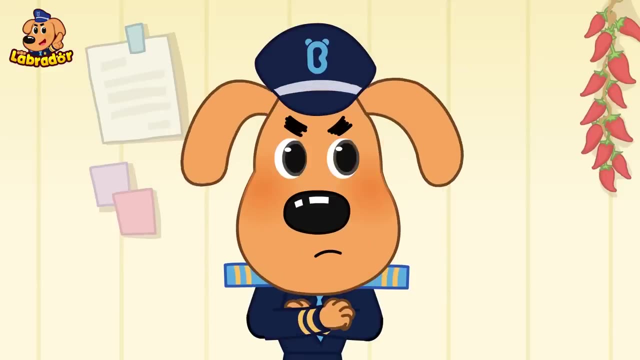 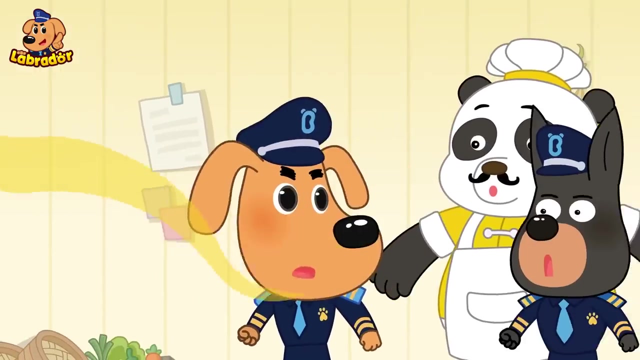 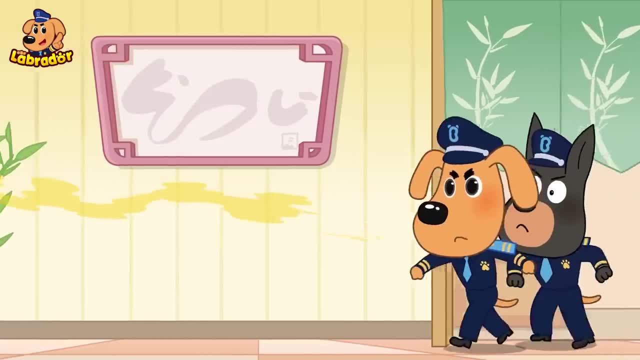 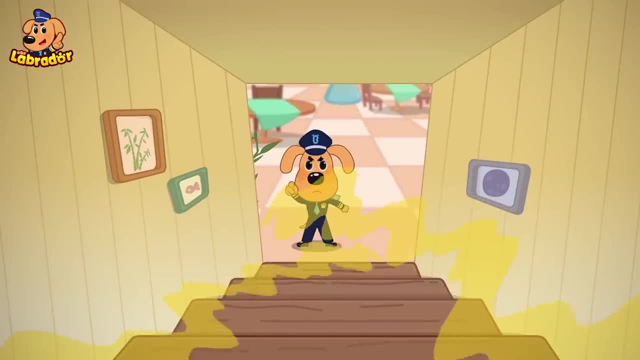 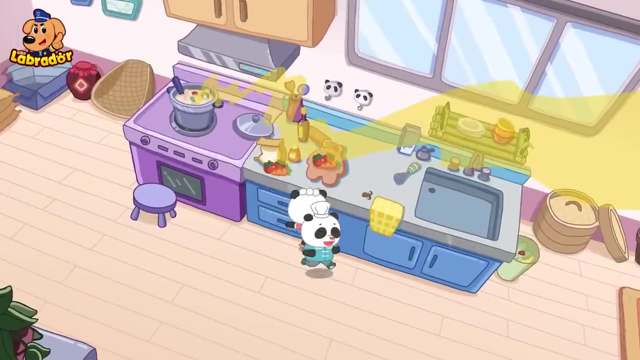 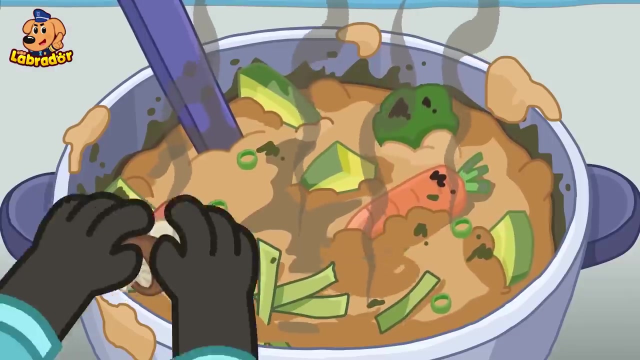 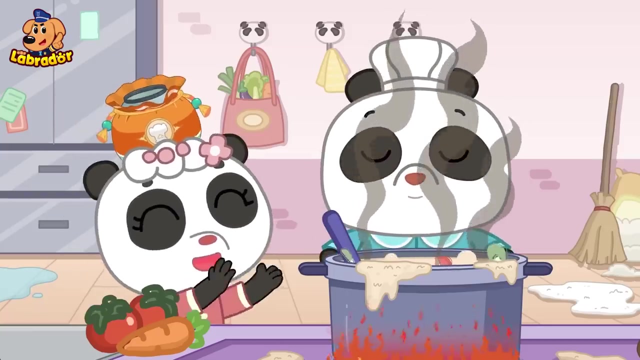 Follow me. The smell's coming from up there. There's another kitchen upstairs. Come on, let's go. Tomato, Carrot, Mushroom, Cucumber- I'm the best chef in the world. Wow, Mr Chef, The secret spice. 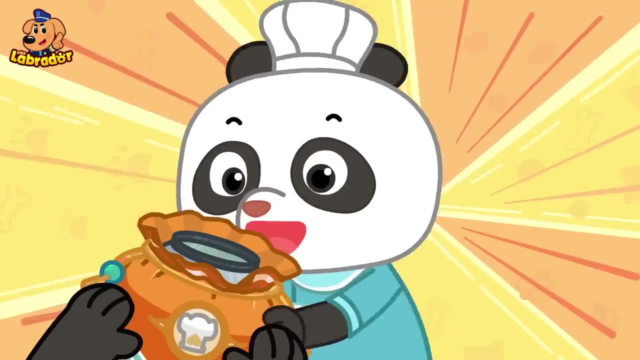 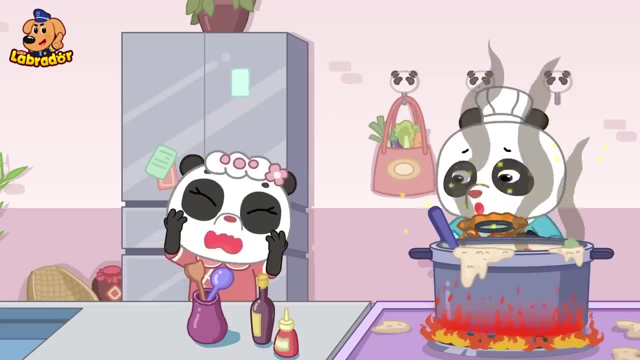 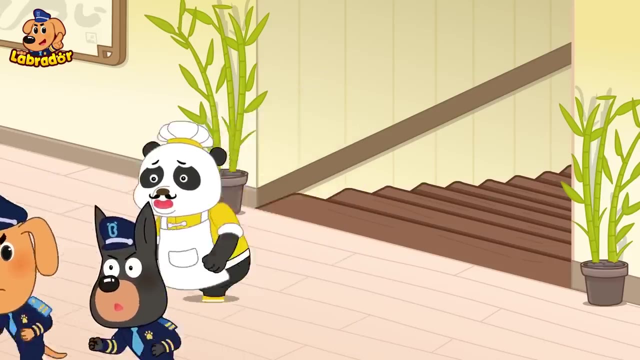 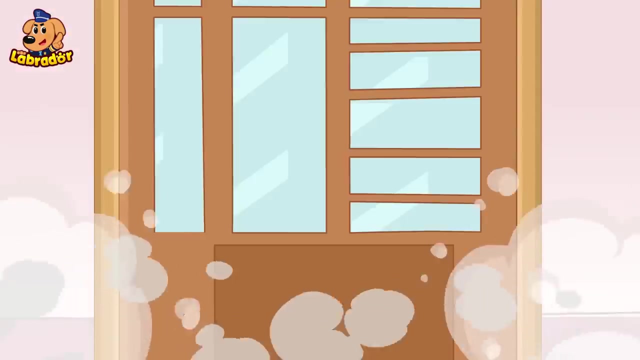 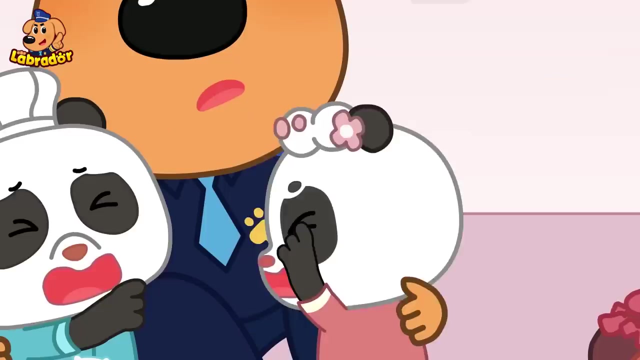 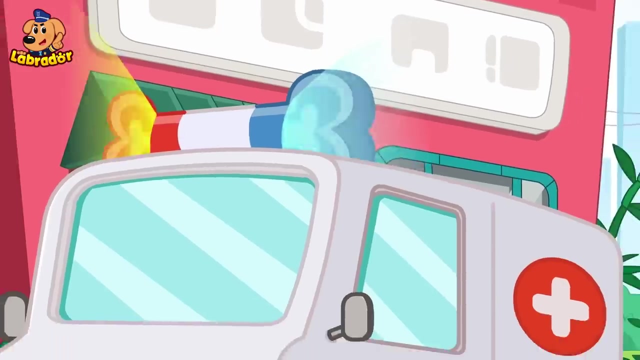 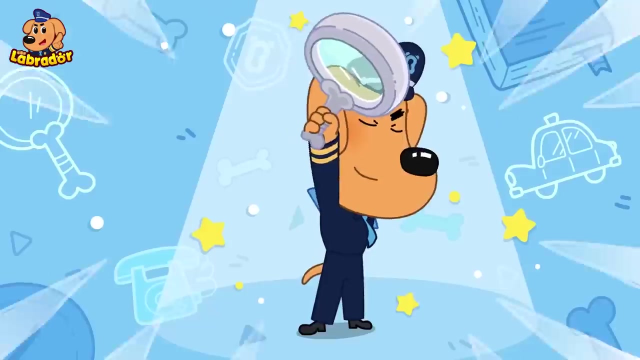 Here, Wow, Ow My eyes. It's my daughter Hurry, Ah, Ah, Watch out My eyes. We need to send her to the hospital right now. Sheriff Labrador's Safety Talk. Kids never play in the kitchen. 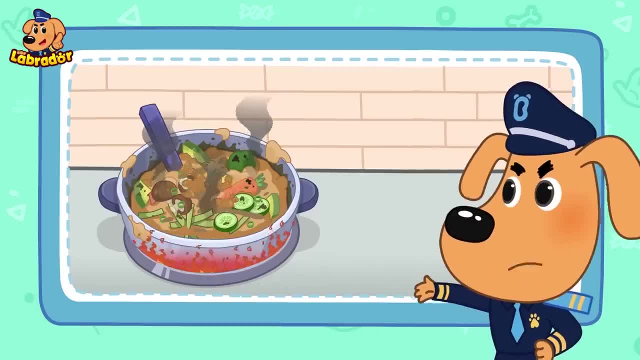 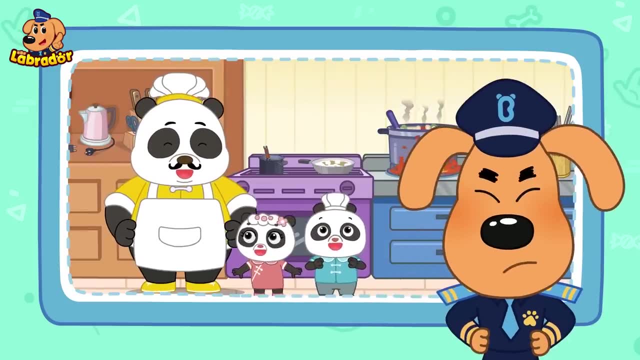 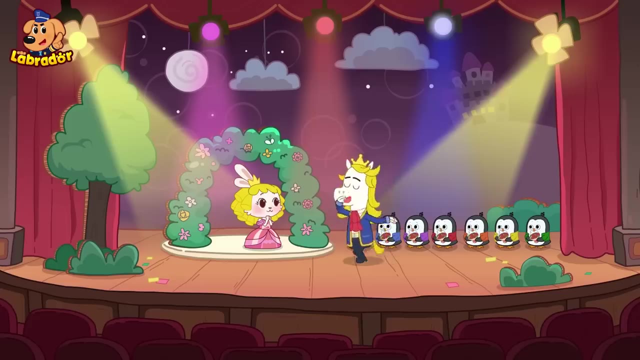 There are sharp knives and tools, boiling water and electric appliances in the kitchen, and they can hurt you Also. parents need to keep an eye on their children when they're in the kitchen too. Woof, My dear Snow White, will you marry me? 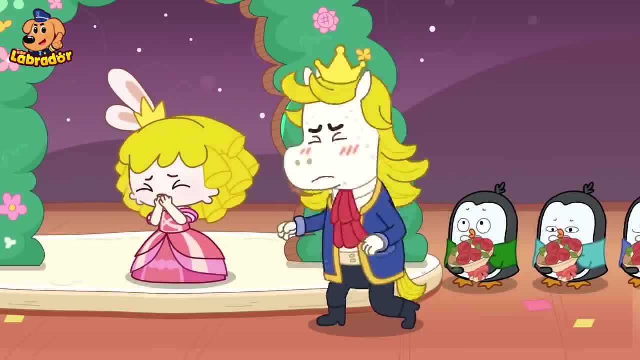 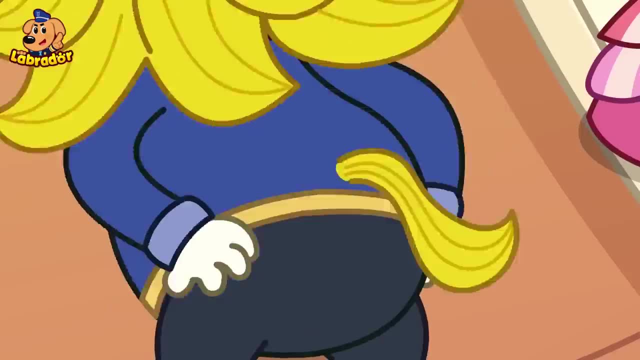 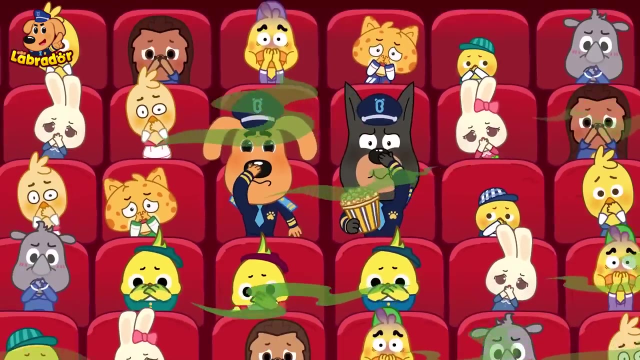 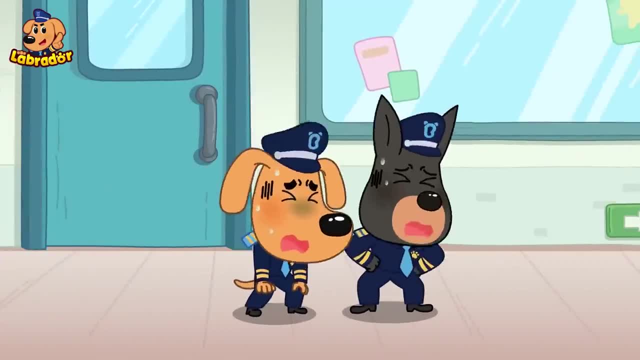 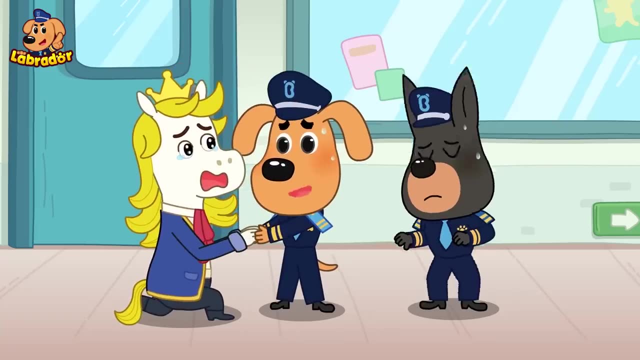 Ah, Ah, Ah, Ah Ah, Sheriff Labrador. Ah, Mr White Horse, Help me. please Calm down, Mr White Horse. What's going on? Someone must have set me up. That's why I keep farting. 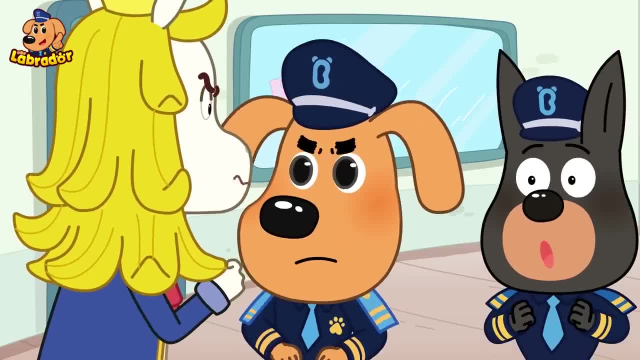 What? Please find out who did this. Don't worry, There's no case that I can't solve. Huh, It was him who set me up, Chef Elephant. I was totally fine before I went on stage, But I had diarrhea after eating your food. 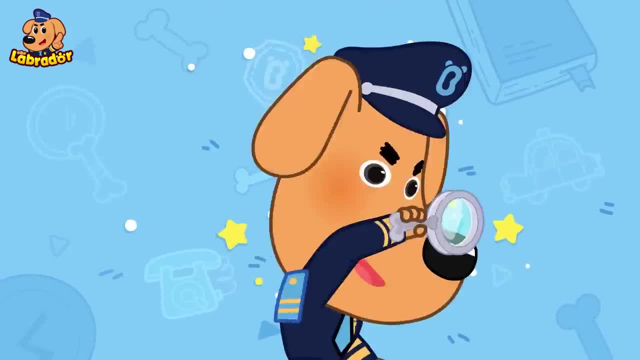 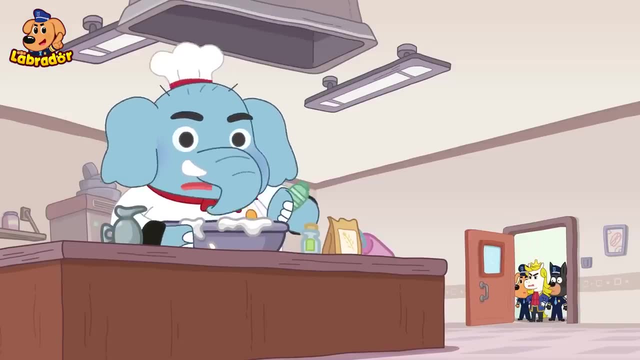 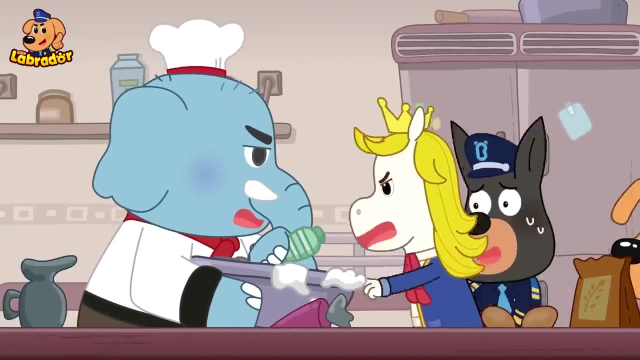 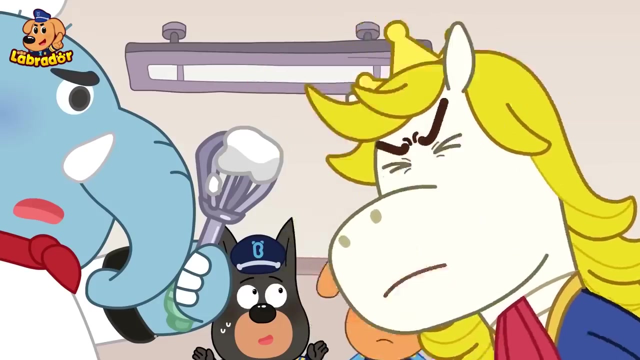 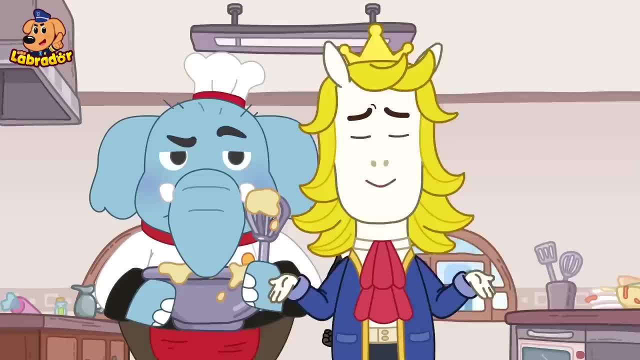 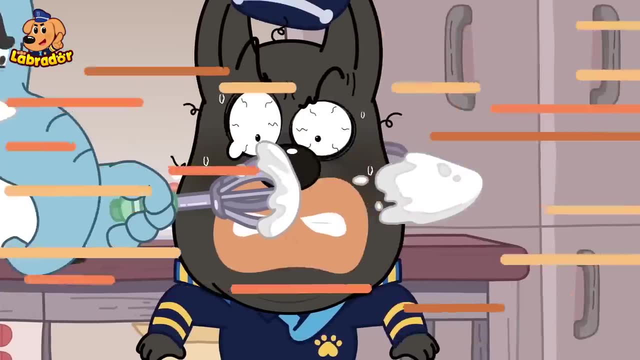 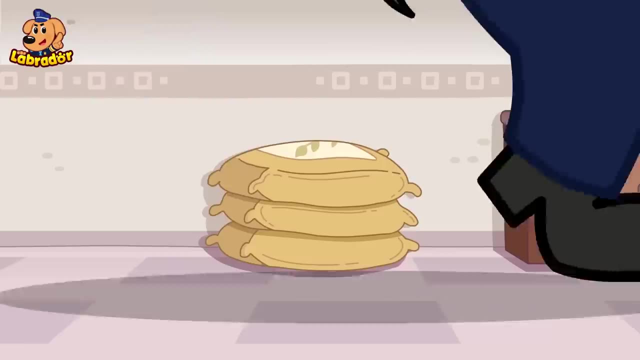 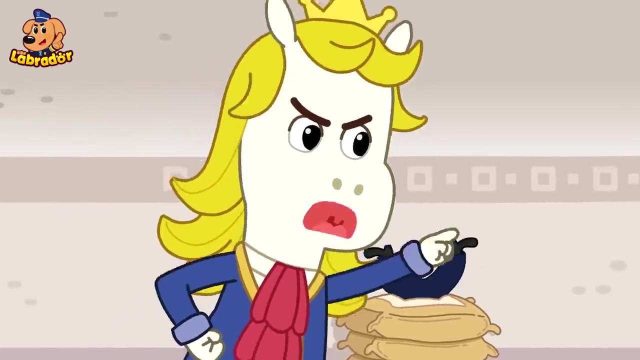 That's the reason why I have diarrhea. You must be jealous of my handsome face… And that's why you have set me up. What are you talking about? Ah, Ah, Ah, Johns, Oh, Oh, Elephant, Are you trying to attack me? Please arrest him. 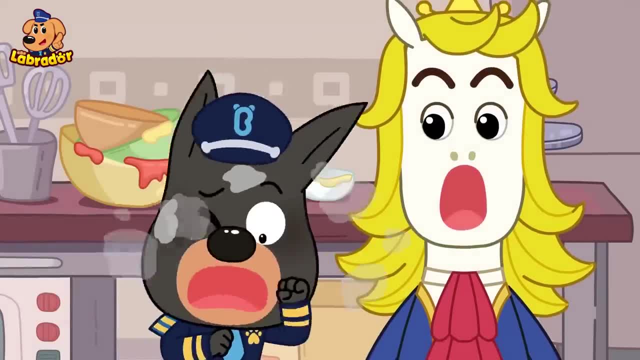 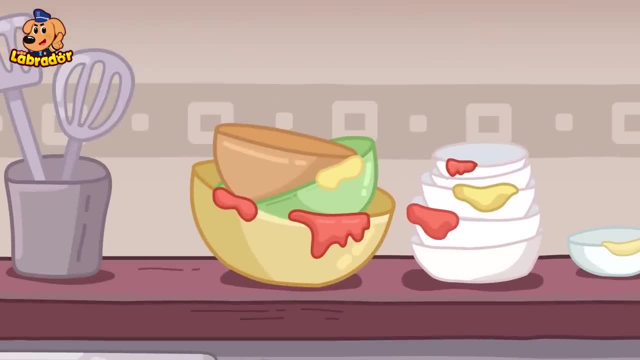 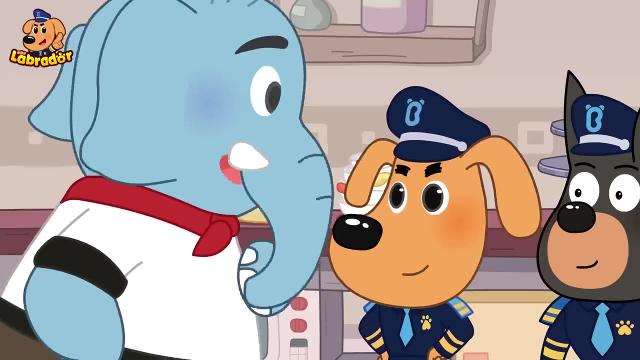 Wait, It wasn't, Mr Elephant. What? Look at the plates over there. A lot of people ate the cake, But you're the only one who got diarrhea. That means there's nothing wrong with the cake. Exactly, Sheriff Labrador made a good point, didn't he? 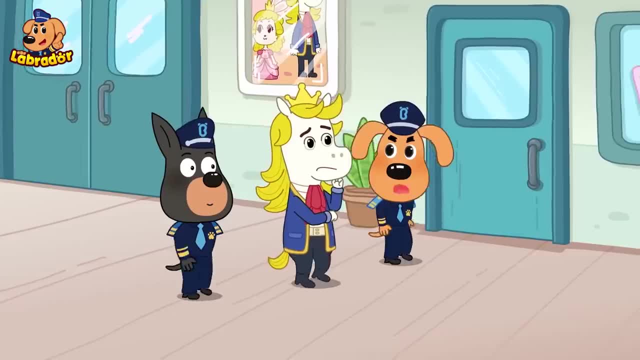 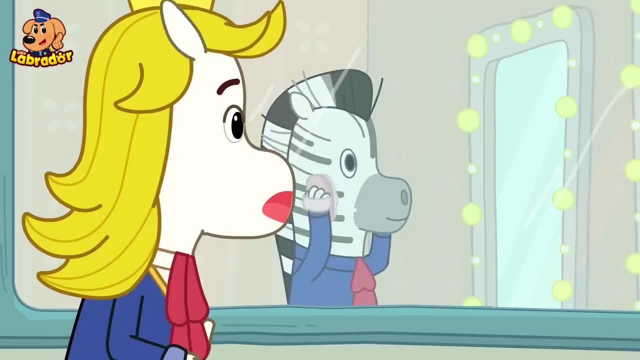 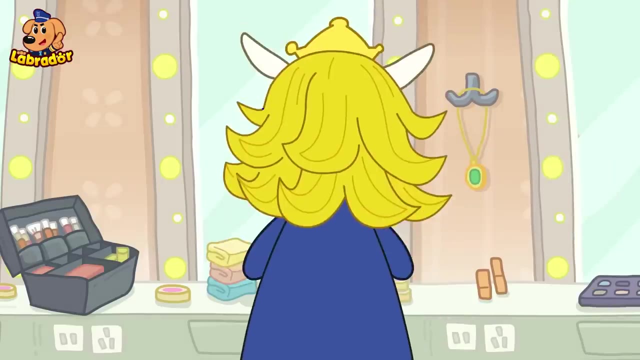 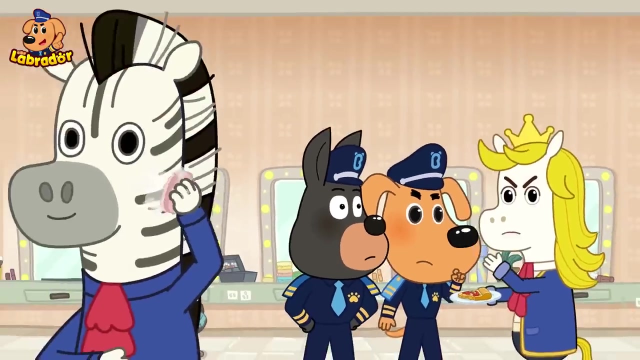 Hmm. Well, Mr White Horse, what else did you eat before you went on stage? Oh, Zebra. Oh, I remember Found it. Mr Zebra gave me a slice of pizza. Look at this, Sheriff Labrador. I'm sure Mr Zebra has put something on my pizza. 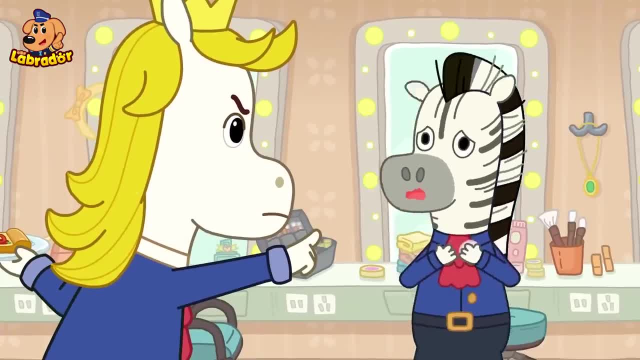 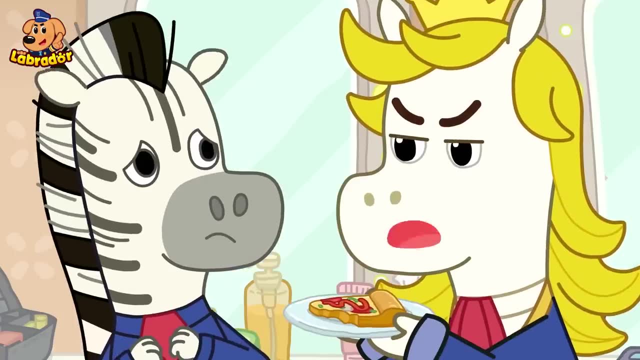 because he wanted to replace me as the prince. What, That's not true? Ha, You were jealous of me, weren't you What? That's why you have put something on my pizza. If I am sick, then you get to play the prince. 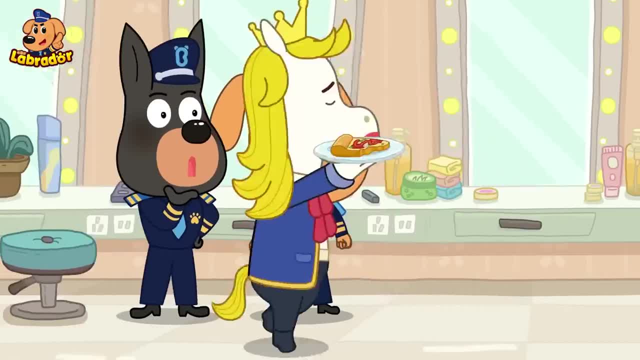 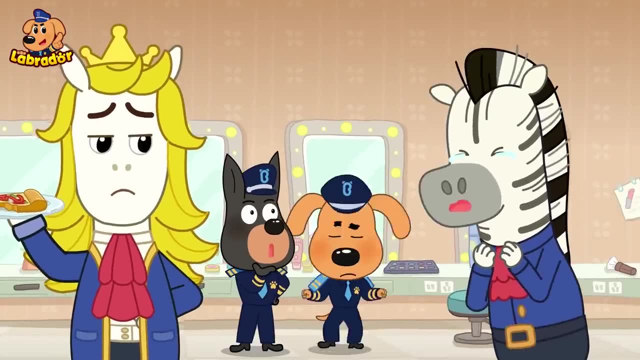 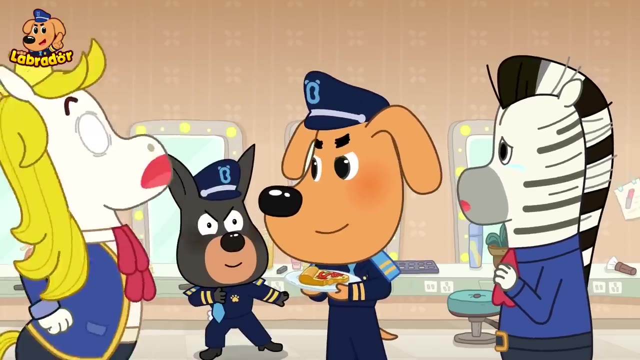 I didn't. I was just born, this handsome. What's wrong with that? I didn't do it. Calm down both of you. We'll find out if there's anything wrong with the pizza Later. Good to me. I can't hold it anymore. 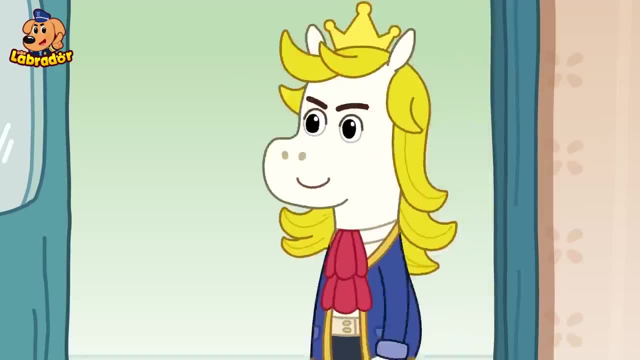 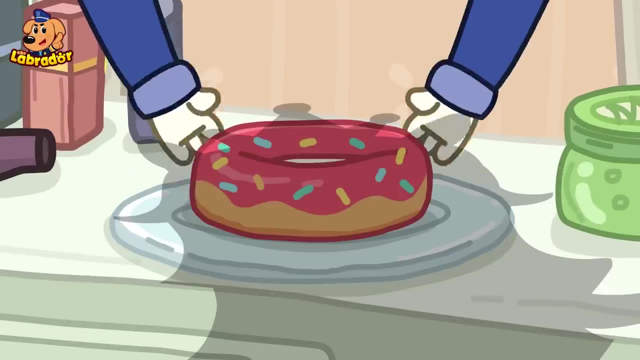 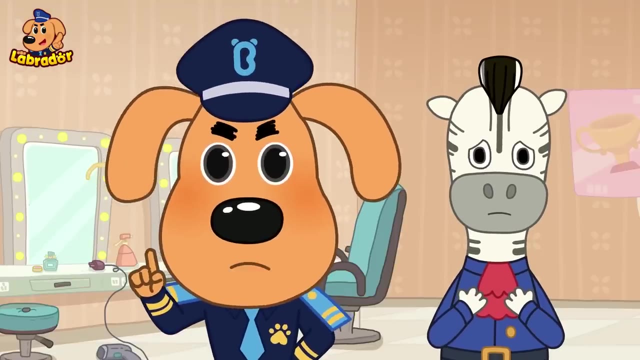 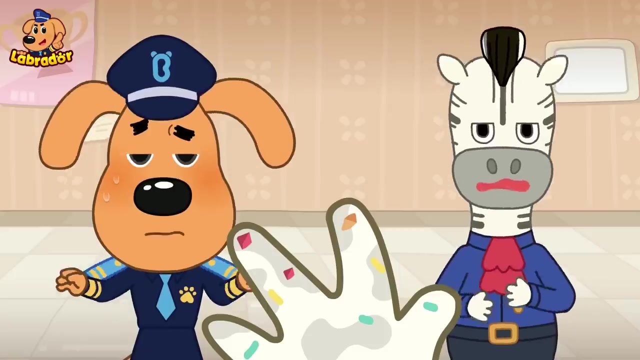 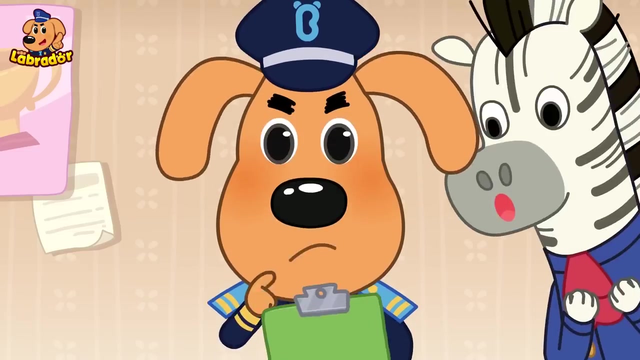 It's okay, I don't need to wash my hands, I'm so hungry. It's a donut, Mr White Horse, you should wash your hands before eating. Oh, It's okay, Not a big deal, Sheriff Labrador, a lot of harmful bacteria were found on the surface of the pizza. 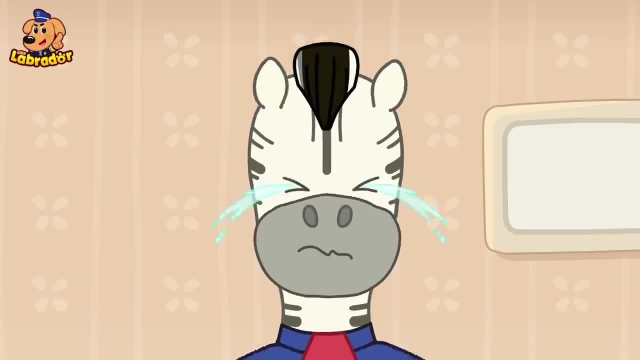 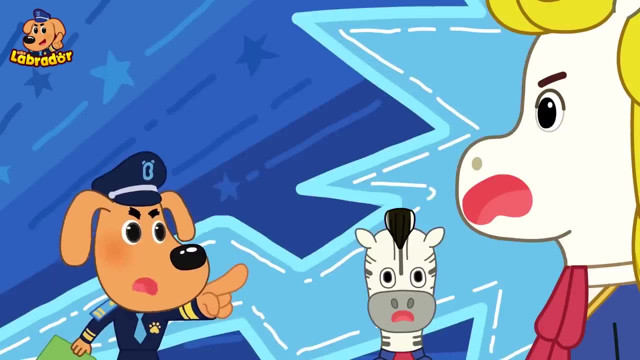 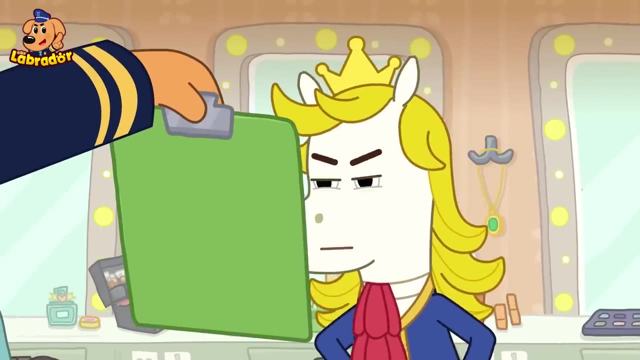 Zebra, it was you. It can't be. It wasn't Mr Zebra. The person who made you get diarrhea is yourself. What, What Me? How can I possibly do that? According to the report, most of the harmful bacteria were found on areas where your fingers have touched. 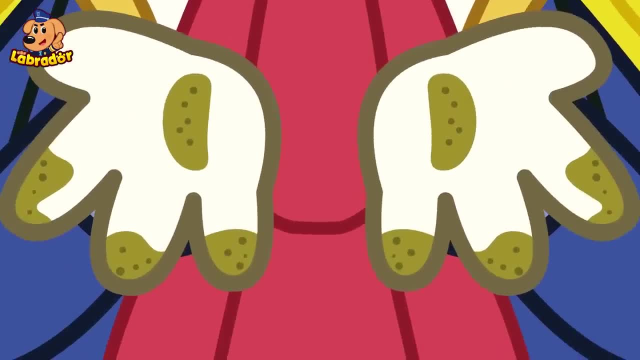 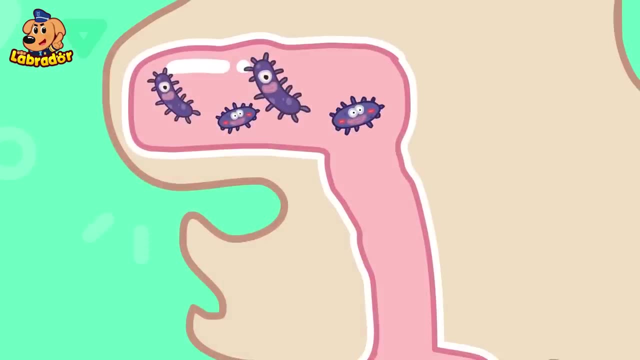 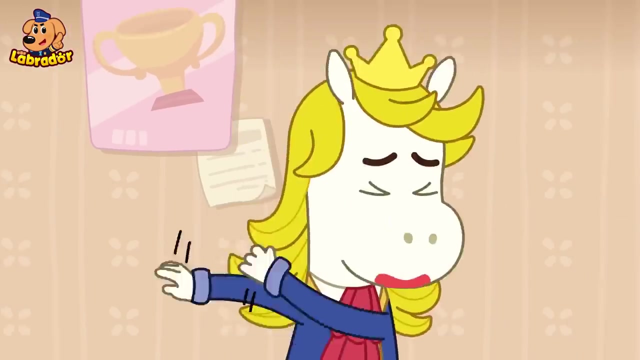 The bacteria were from your hands. You didn't wash your hands before eating the donut just now either. The bacteria on your hands got into your stomach and that's why you had diarrhea. I'm, I'm, I'm, I'm. 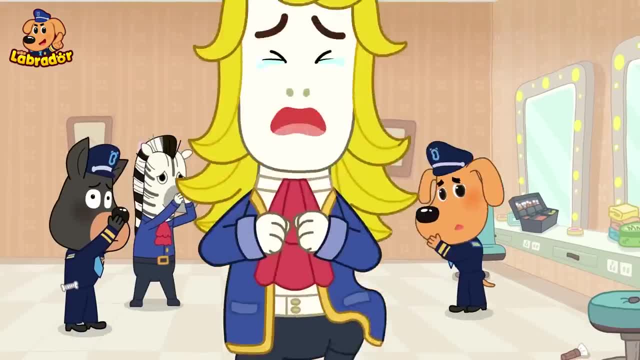 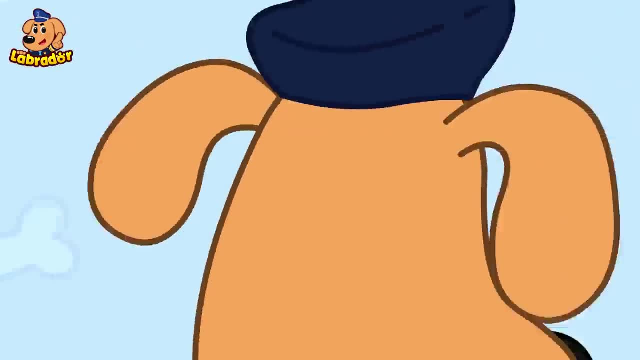 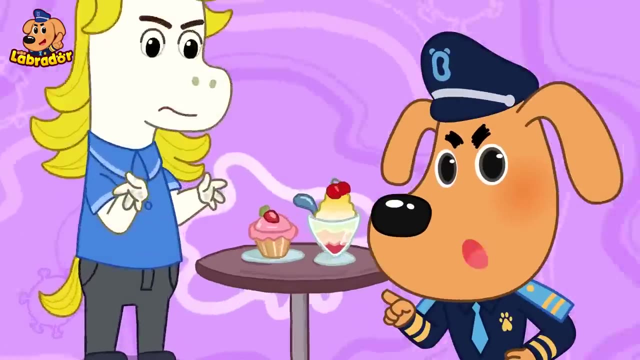 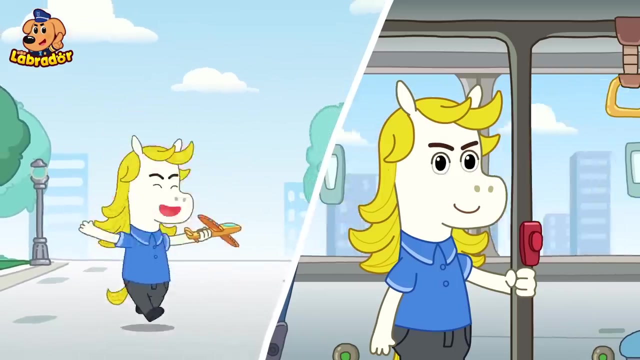 I'm washing my hands right now. I don't want to be the farming prince ever again. Sheriff Labrador's: Safety Talk, Kids. there are lots of bacteria on our hands. Wash your hands before eating, after going to the bathroom, playing outside and using the public transit. 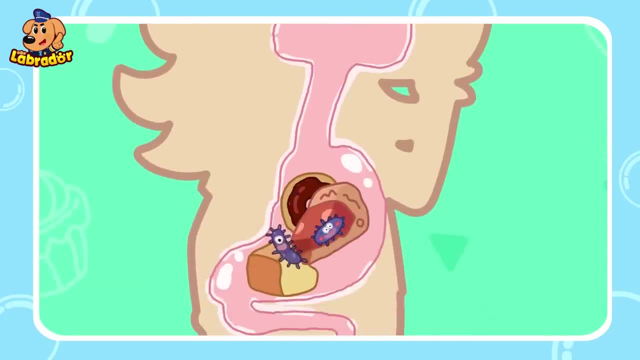 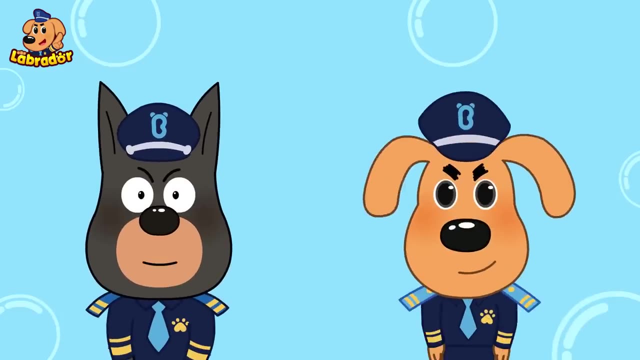 If you don't the bacteria, The bacteria can get inside your stomach and you can get sick. That's why we should regularly wash our hands, Woof.